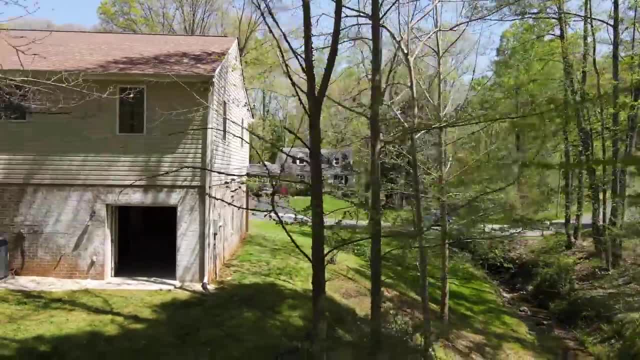 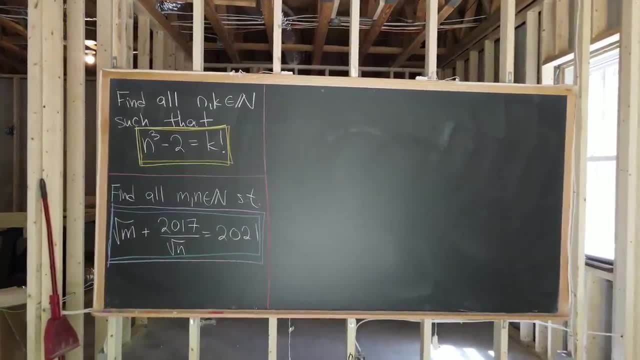 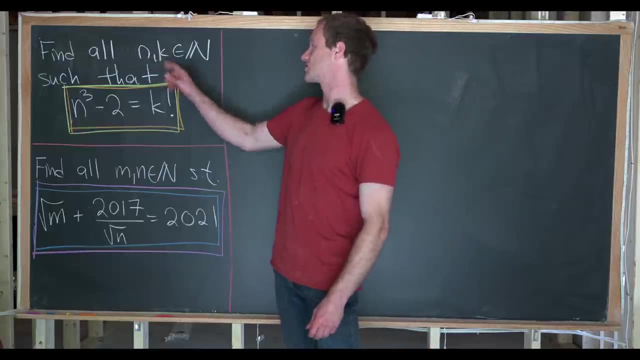 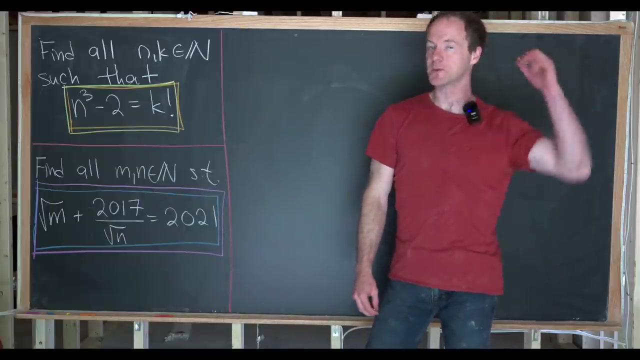 I want to look at two nice number theory problems today. So the first one goes like this: We want to find all natural numbers n and k, such that n cubed minus 2 equals k factorial. We're going to use the notion of congruence modulo m here, And in fact we're going to use the 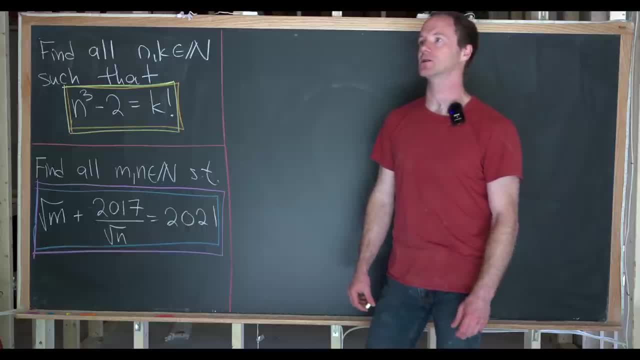 fact that k factorial is always going to be congruent to 0 mod 4 if k is bigger than or equal to 4.. And when I say 0 mod 4, that means it's a multiple of 4.. So let's look. 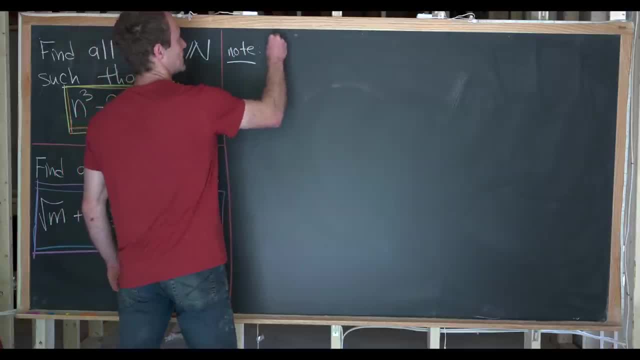 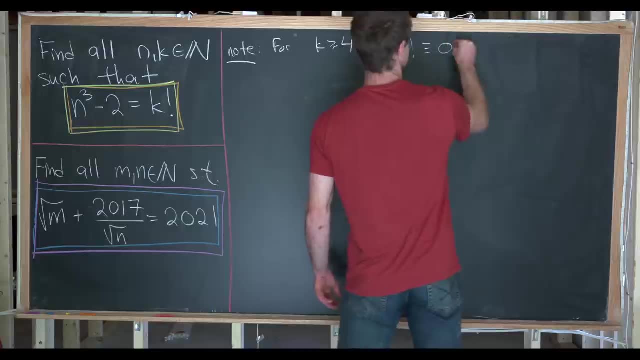 at that. Maybe we'll make that the first thing that we notice. For k bigger than or equal to 4, we have k factorial is congruent to 0 mod 4.. And why is that? Well, if k is bigger than or equal to 4, we have k factorial is congruent to 0 mod 4.. And why is that? Well, if k is bigger than or equal to, 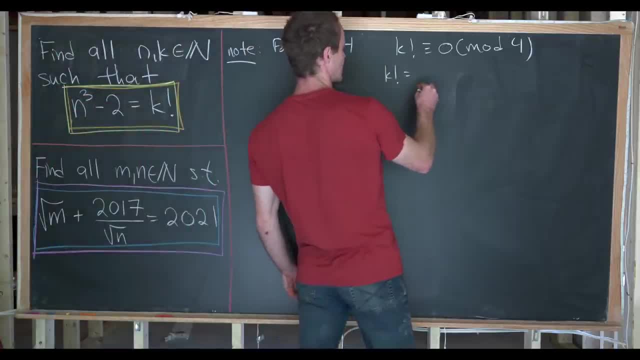 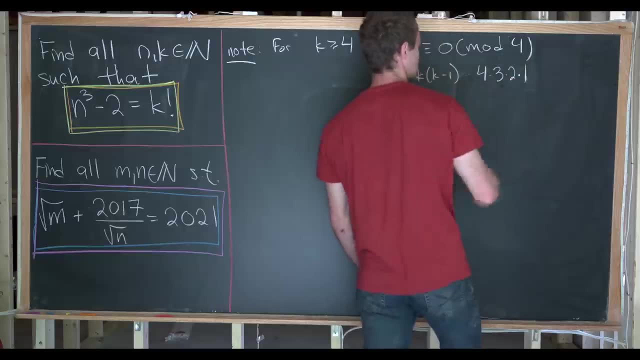 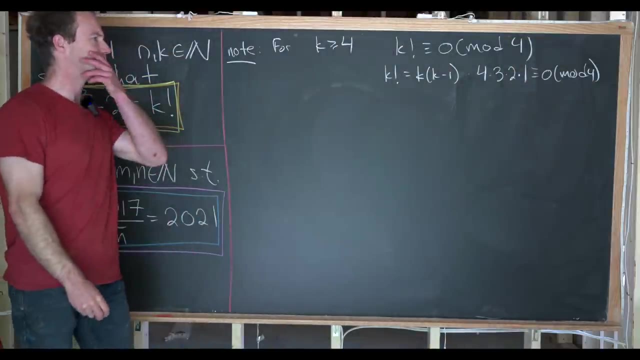 4, then k factorial can be rewritten as k times k minus 1, all the way down to 4 times 3 times 2 times 1, which is clearly a multiple of 4.. We've got a 4 right there, Okay, So. 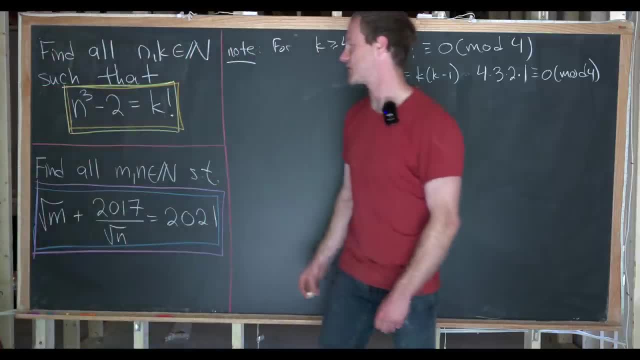 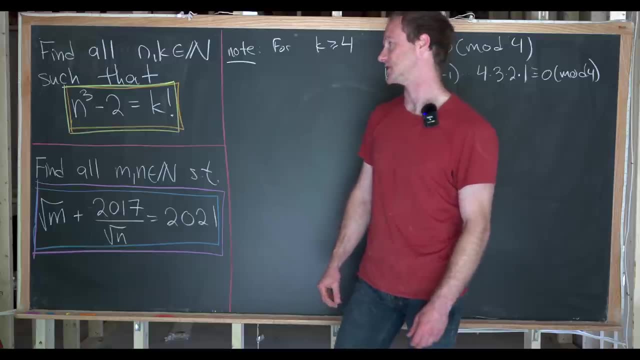 next up, we want to look at the possible perfect cubes modulo 4.. And notice that that's really going to restrict our possibilities for solutions. So I'm just going to make a little bit of a chart and I'll look at values of n and. 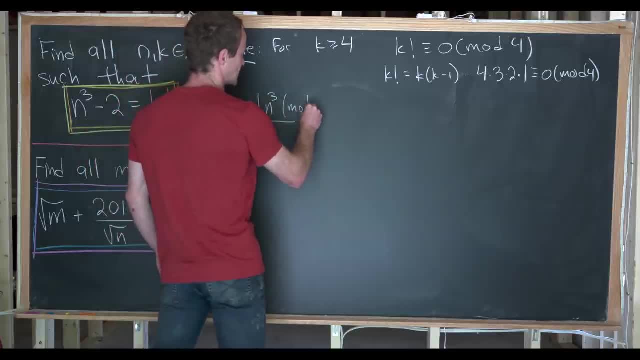 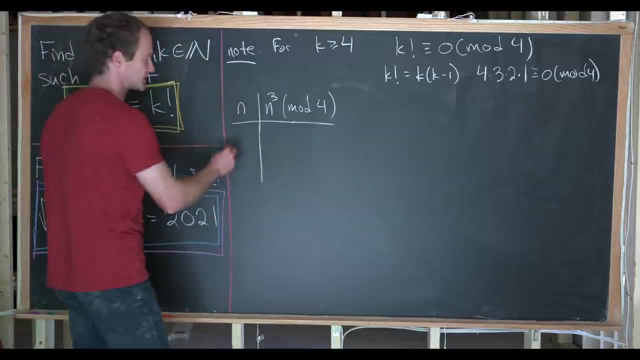 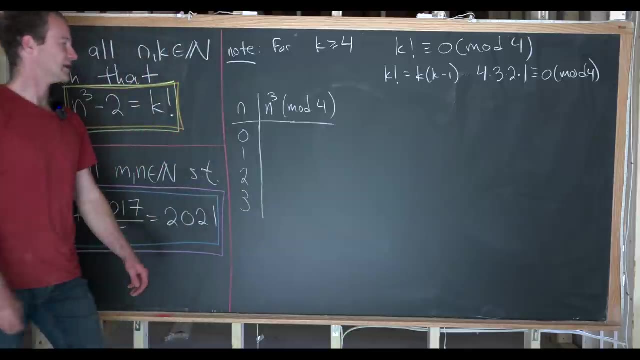 then I'll look at values of n cubed modulo 4.. Okay So, since I'm working mod 4, I only need to look at 4 numbers, really 4 equivalence classes, That's 0,, 1,, 2, and 3.. Now let's. 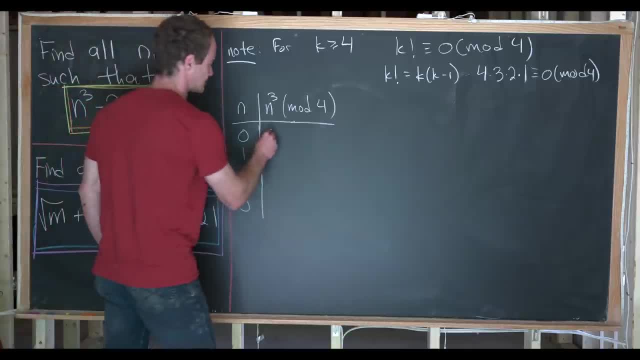 see what we get: 0 cubed is going to be 0 mod 4.. In other words, if n is a multiple of 4, then k is greater than or equal to 4.. So that's really going to restrict our 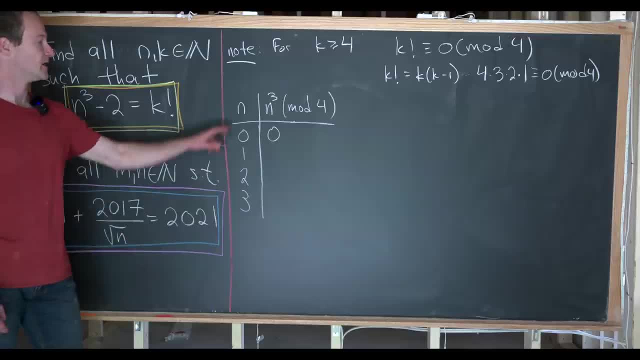 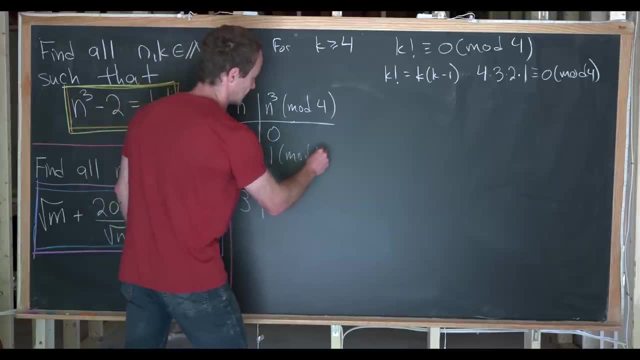 possibilities for solutions. So if n is a multiple of 4, then n cubed is a multiple of 4.. So if n is congruent to 1 mod 4, then n cubed is also congruent to 1 modulo 4.. If 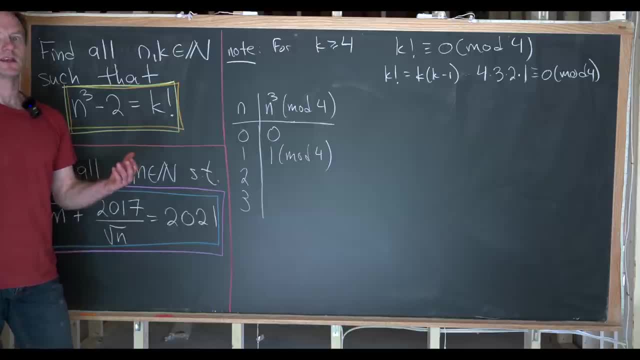 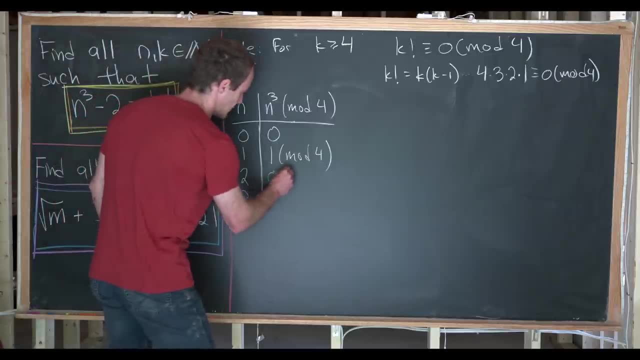 n is congruent to 2 mod 4, then n cubed is congruent to 8 mod 4.. 2 cubed is 8, but 8's a multiple of 4, so we get 0 mod 4 here. Okay. And then finally, if n is congruent to 3 mod, 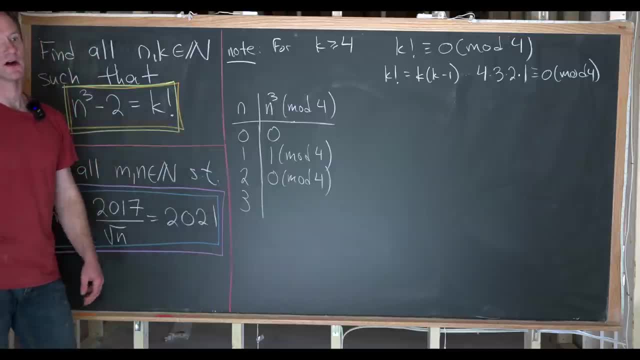 4, then n is congruent to 1 mod 4.. So that's really going to restrict our possibilities for solutions. So if n is congruent to 1 mod 4, then n cubed is also 3 mod 4.. And we can. 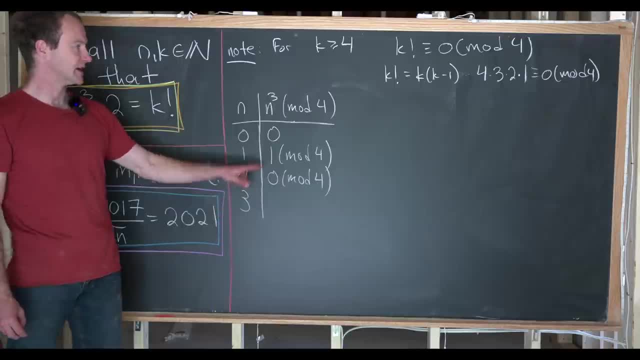 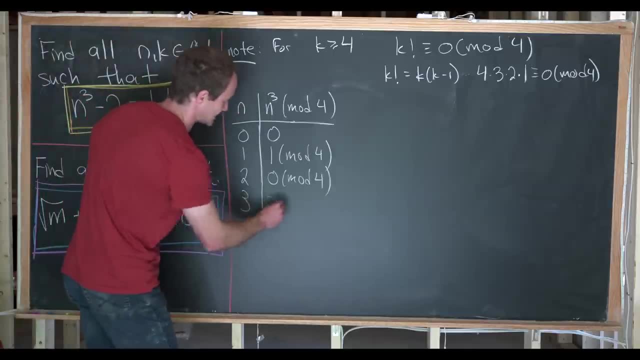 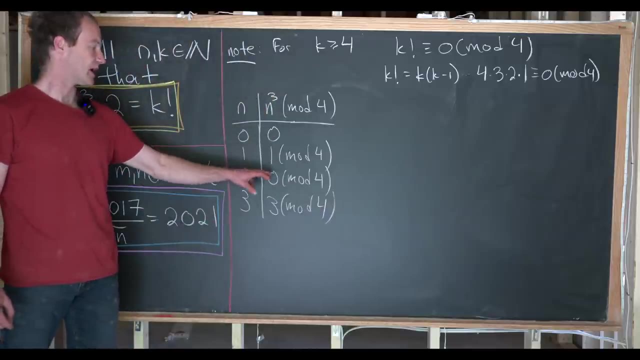 actually see that very quickly by seeing that 3 is congruent to negative 1 mod 4.. But if we take negative 1 cubed, we get negative 1. But again, that's the same thing as 3 mod 4.. Now, next up, I want to notice that these are the only possible perfect cubes: mod 4.. 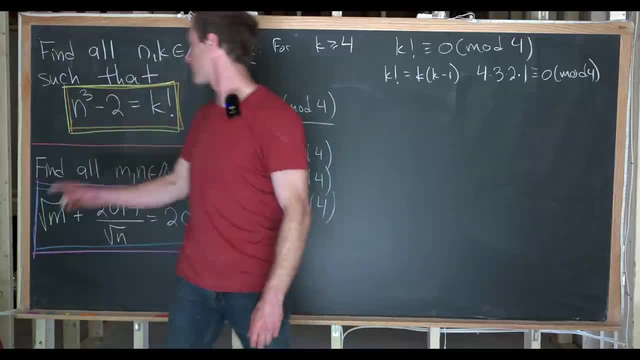 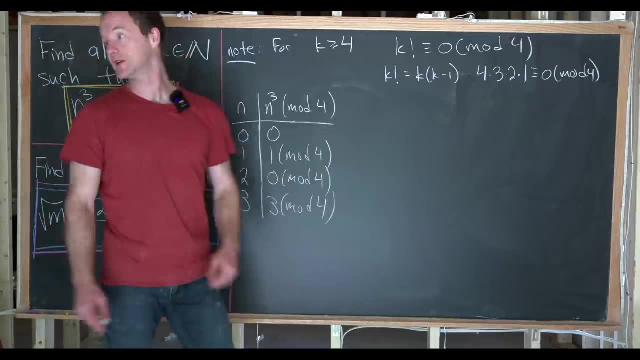 We have 0,, 1, and 3.. But in order for this to be solvable, when k is bigger than or equal to 4, we would need n cubed to be congruent to 2 mod 4.. So this statement right here. 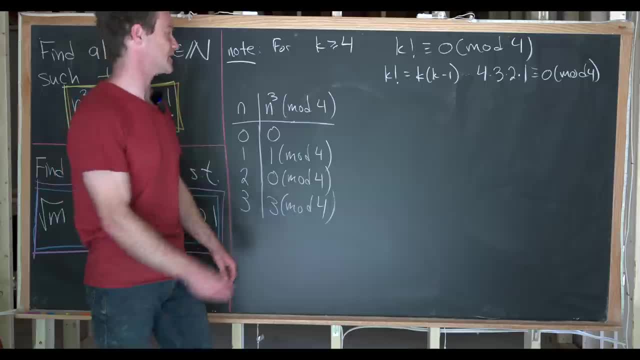 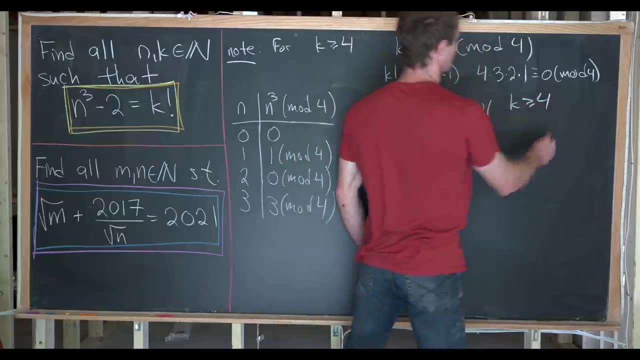 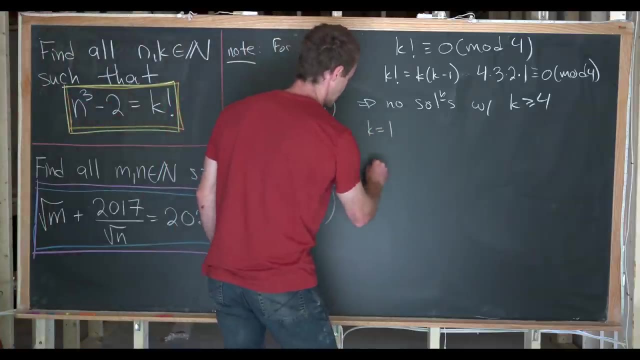 or this chart right here, and this observation right here implies that there are no solutions with k bigger than or equal to 4.. But that means we just need to check a couple of values of k. We'll look at k equals 1,, we'll look at k equals 2, and then we'll finally look at the. 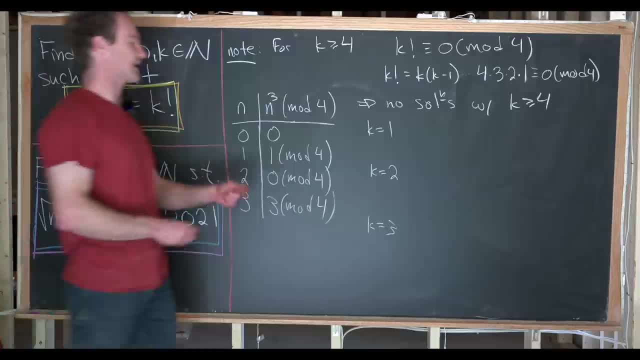 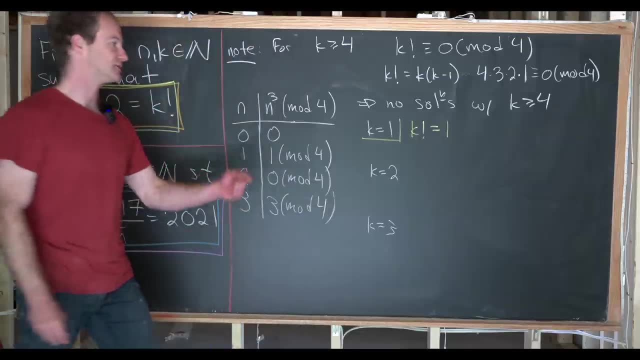 k equals 3 and see what we get. So for k equals 1, we have k factorial equals 1 factorial, which is 1.. Which means we need to solve the equation: 1 equals n cubed minus 2.. But let's 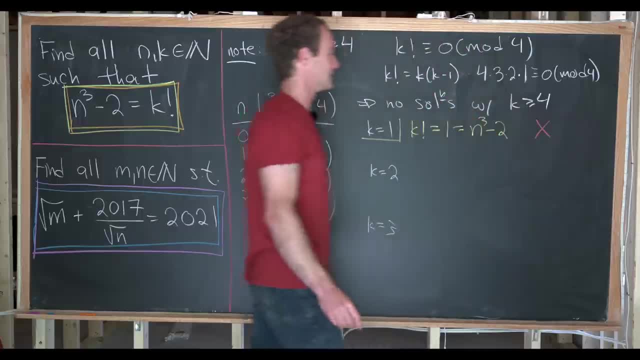 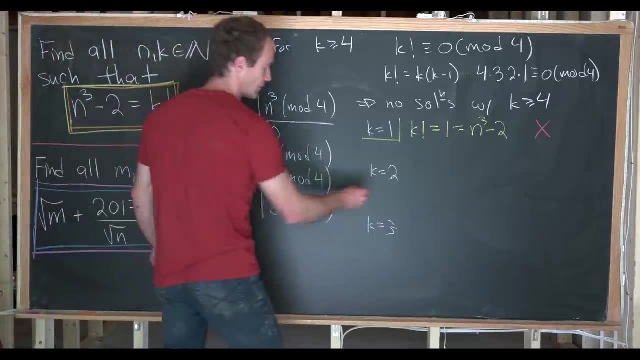 notice that there's kind of obviously no solution to that. That's because, in order for there to be a solution, 3 would have to be a perfect cube. Now let's see what we get here If k is equal to 2.. 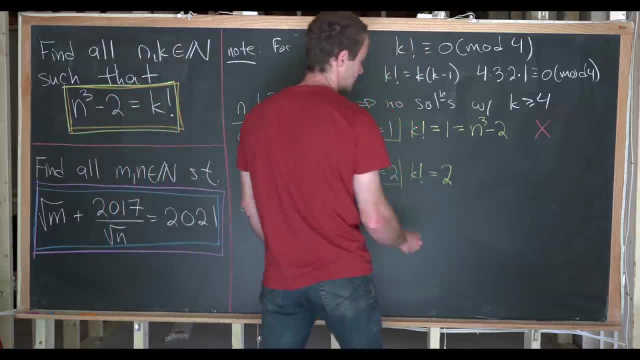 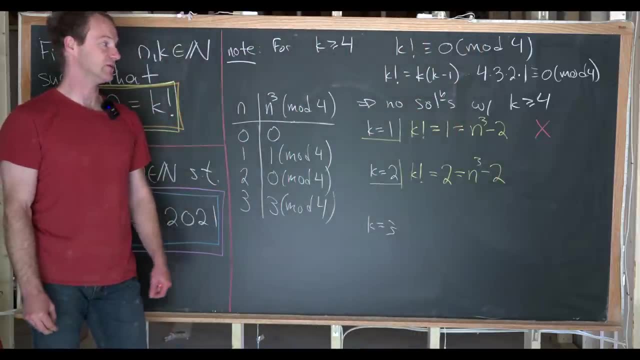 then that makes k factorial equal to 2, but now we need to solve: 2 equals n cubed minus 2.. But again, n cubed minus 2 equals 2 has no solution. If it did, then 4 would be a perfect cube. 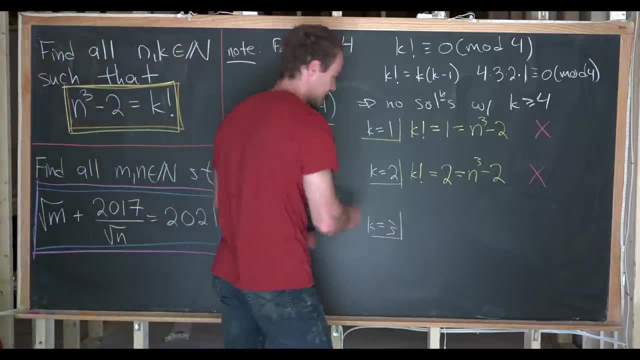 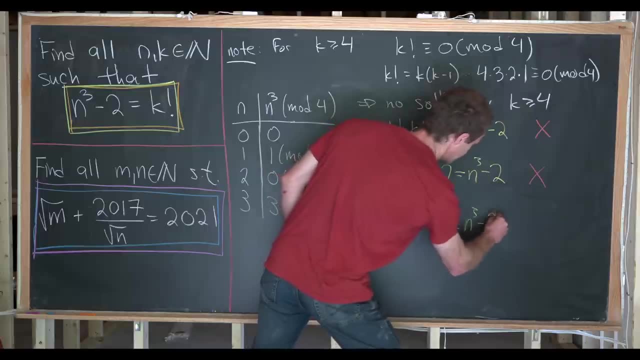 Then, finally, if k equals 3, then k factorial equals 6,, which means we have the equation 6 equals n cubed minus 2, which is the same thing as saying n cubed equals 8, which is the same thing as saying n equals 2.. 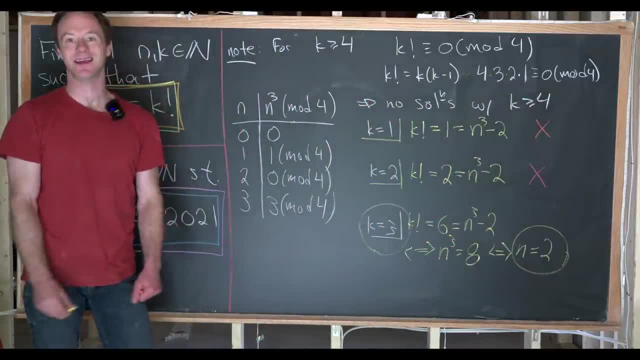 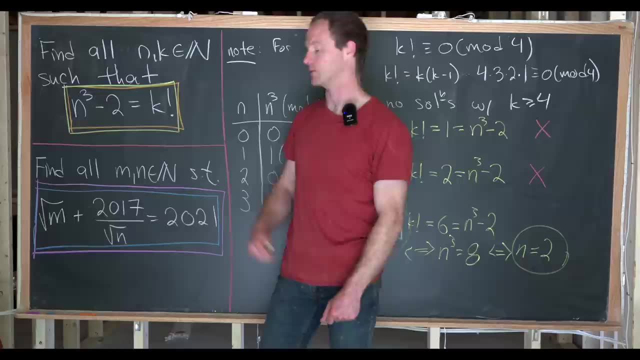 So there we have our solution: k equals 3 and n equals 2, and that's the only such solution. Okay, let's get rid of this, and then we'll look at our second problem. So let's look at the second question. 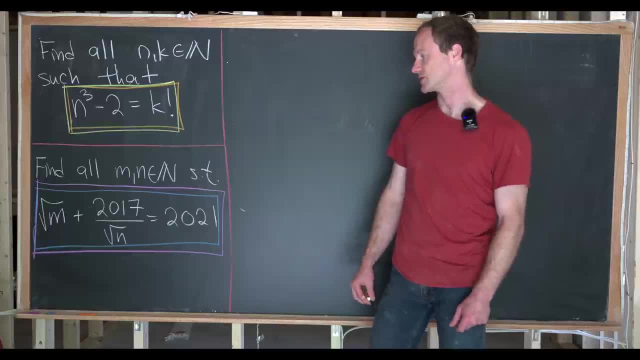 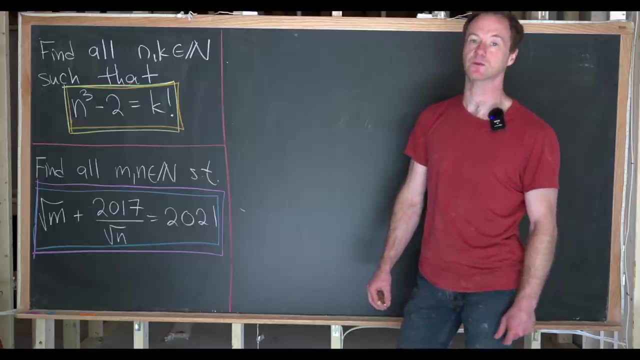 We want to find all m and n, which are again natural numbers, such that the square root of m plus 2017 over the square root of 2 of n equals 2021.. Okay, so the first thing I'd like to do is rearrange this. 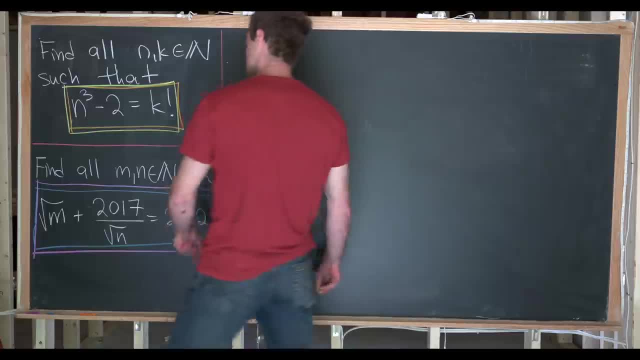 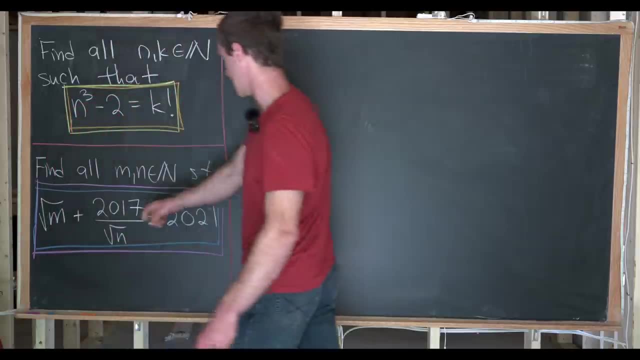 so I can get rid of the square roots as much as possible. So let's see how we can do that. We can rearrange this so we have: 2017 over the square root of n equals 2021 minus the square root of m. 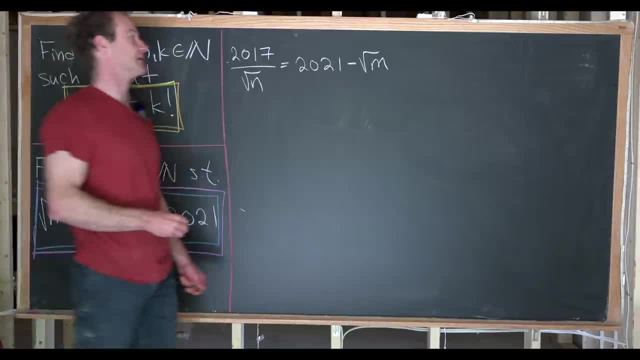 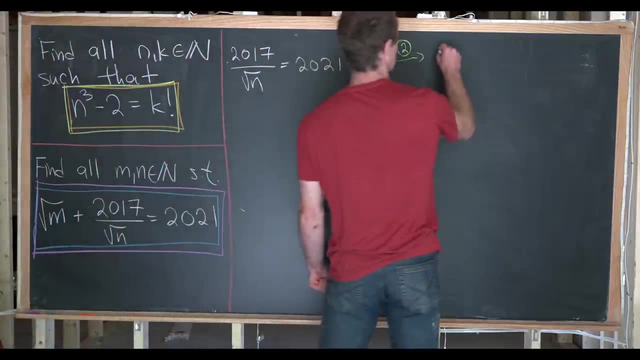 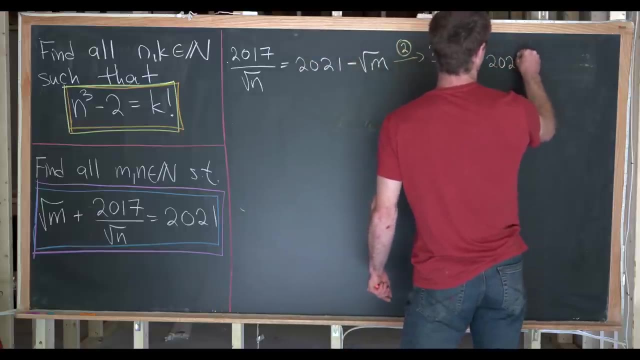 So I've just moved that square root of m to the right-hand side, But now I can square this entire equation and on the left-hand side that's going to give me 2017 squared. I'll just write it like that: over n equals 2021 squared minus 4,042 times the square root of m plus m. 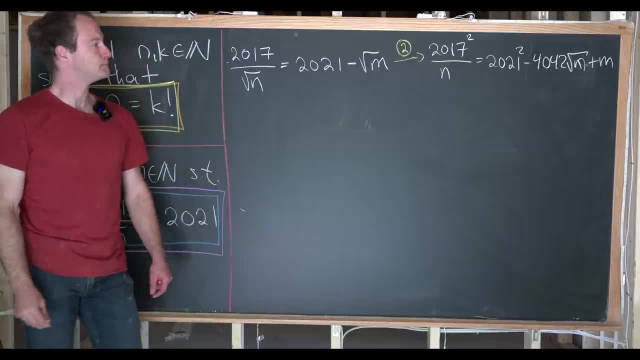 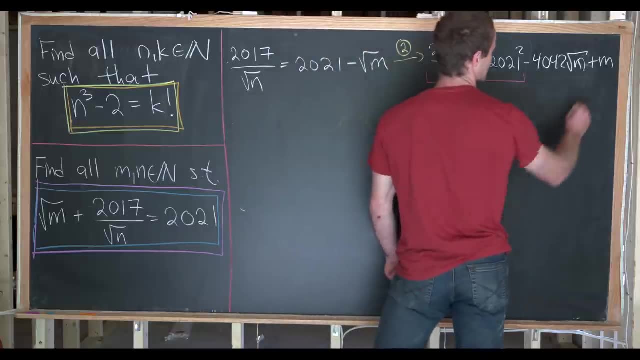 So that's just from squaring that binomial. But now I want to notice that this guy right here is a rational number. This guy right here is a rational number and this guy right here is a rational number. Some of those are obviously natural numbers. 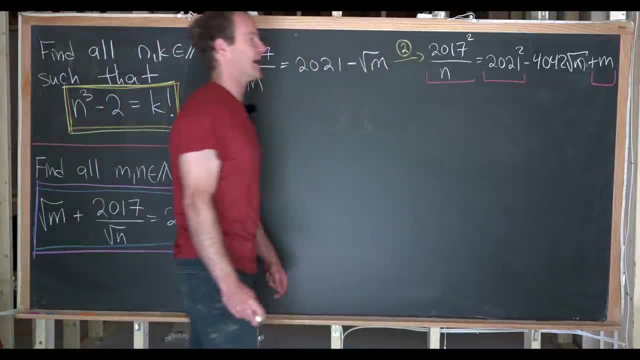 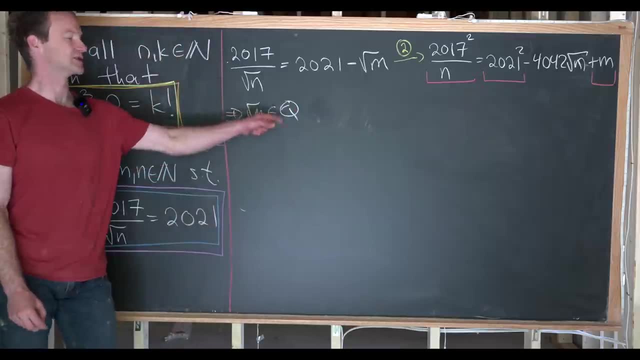 But that implies that what's left over also has to be a rational number. In fact, that means that the square root of m is a rational number. But then, if the square root of m is a rational number, it's well known that that means that the square root of m is in fact a natural number. 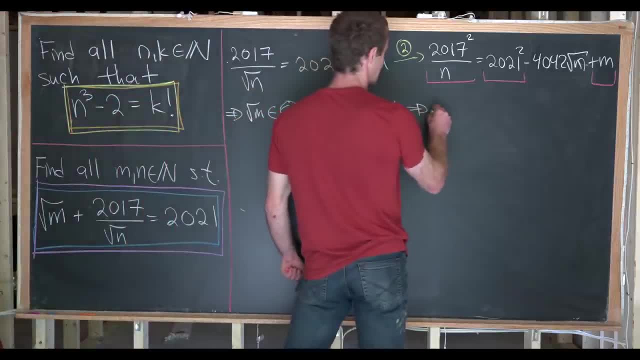 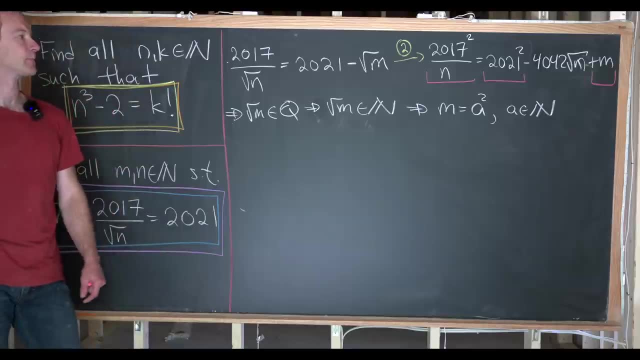 But if the square root of m is a natural number, that means m is a perfect square. Let's write it as a squared for some natural number, a like that. Okay, sweet, Now let's go ahead and take that and plug it into our original equation. 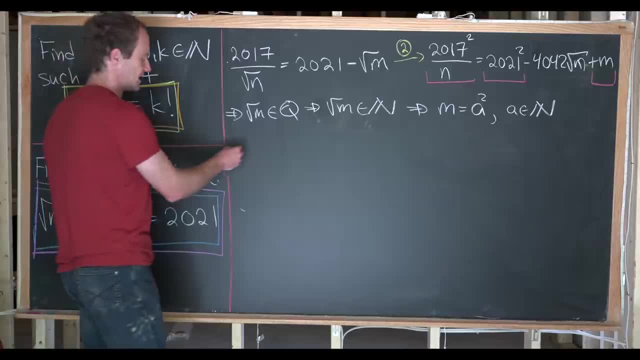 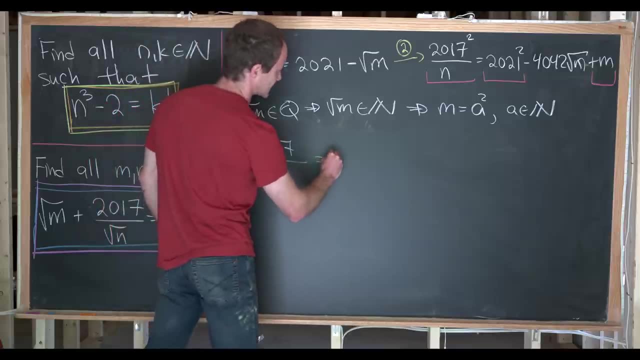 Well, really this rewritten original equation and see what we end up with. So that tells us that 2017 over the square root of n equals 2021 minus the square root of a squared, But that's going to be m squared. 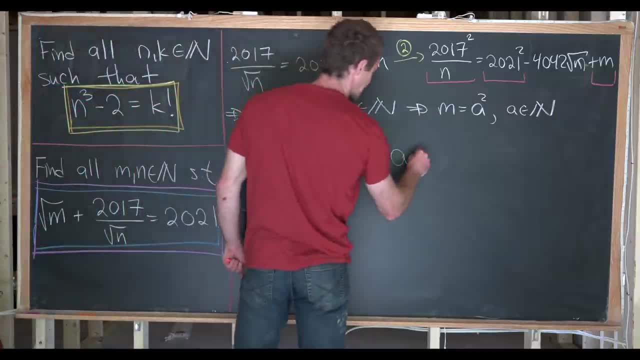 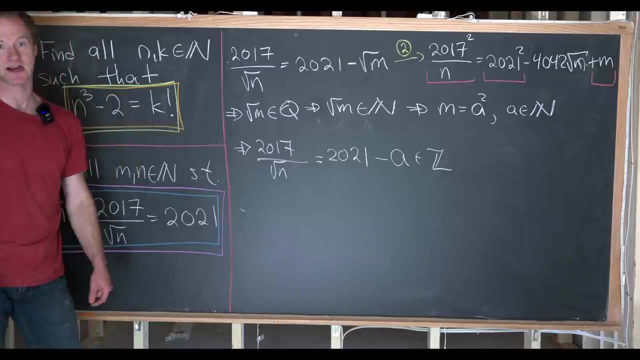 That's going to be minus a. But now notice that this entire right-hand side is most definitely an integer. But if the right-hand side is an integer, that means the left-hand side is an integer. But if the left-hand side is an integer, that means well, really two things. 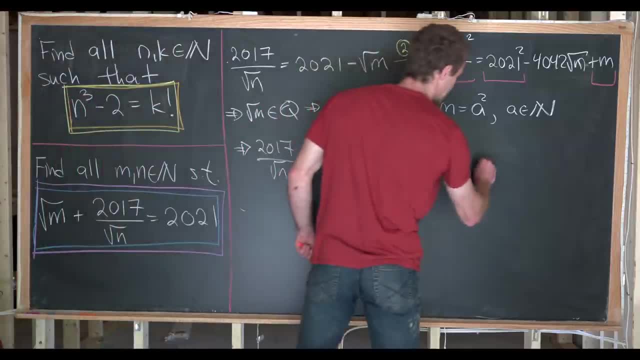 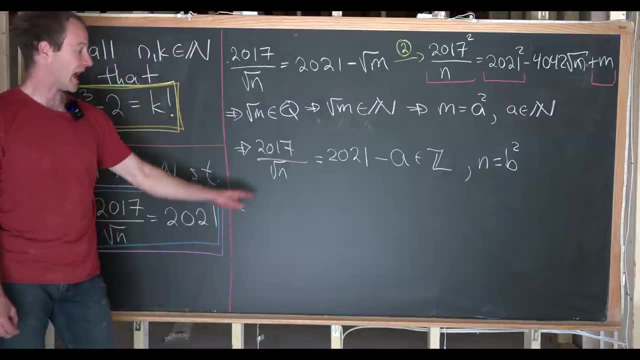 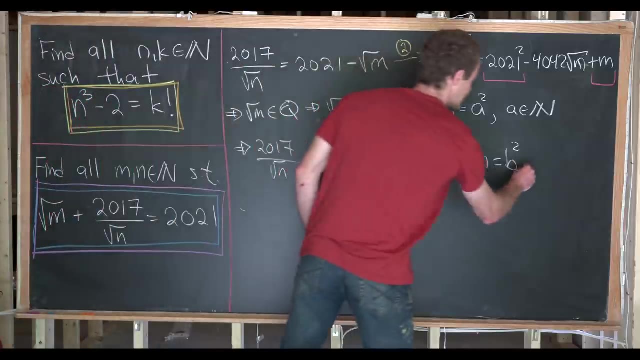 n is a perfect square, So we could write that down real quick. n equals b, squared, kind of with a parallel argument to what we did with m, And, And The square root of n divides 2017.. But notice that the square root of n now is just b. 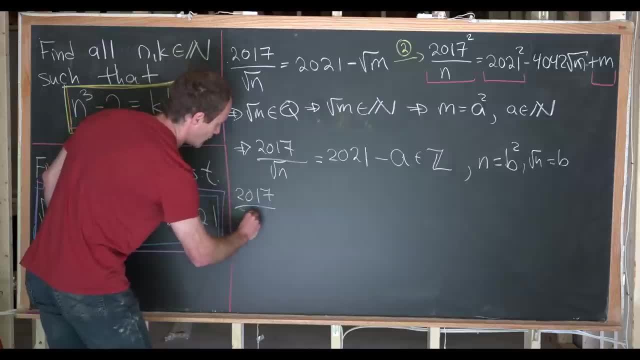 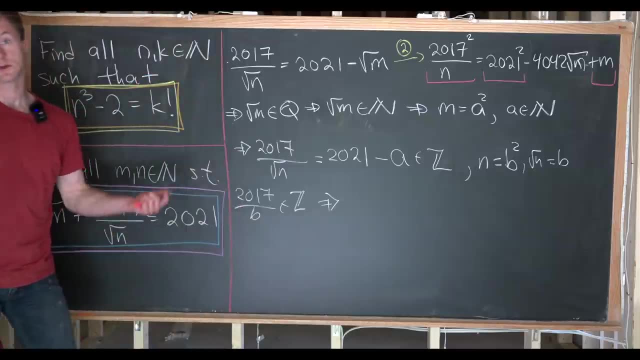 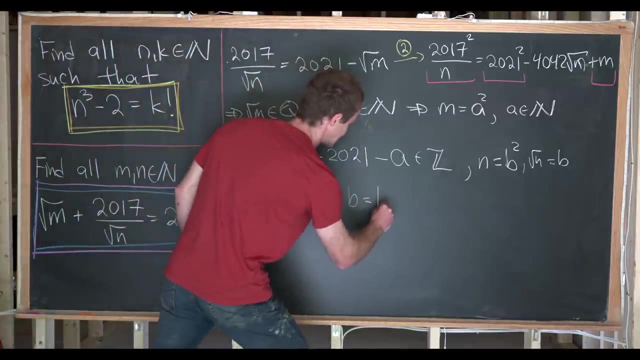 So we have 2017 over. b is an integer, But 2017 is prime, So you can check that. It's not too hard to check. The fact that 2017 is prime tells us that b has to be equal to 1 or 2017.. 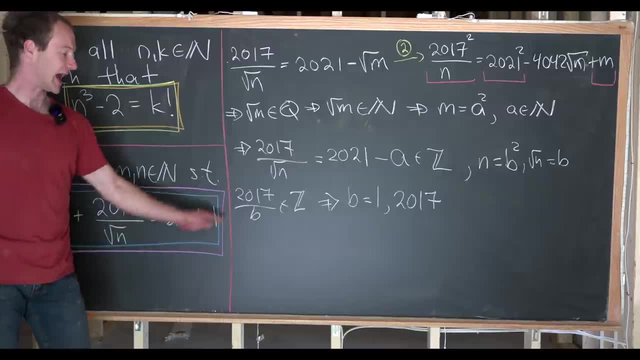 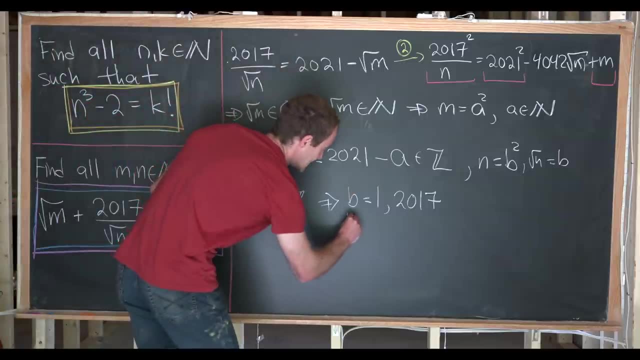 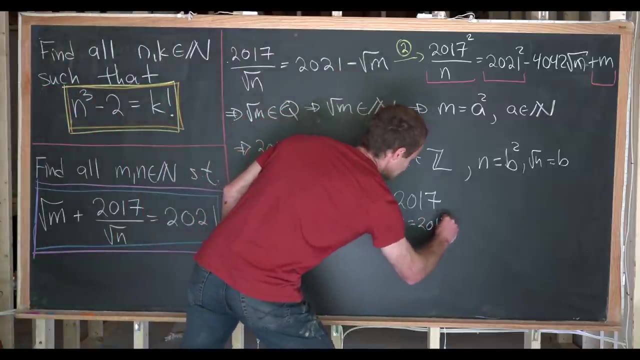 That's the only way we can get an integral value out of this quotient. Okay, So if b equals 1, notice that that means that n equals 1.. If b equals 2017, that means that n equals 2017 squared. 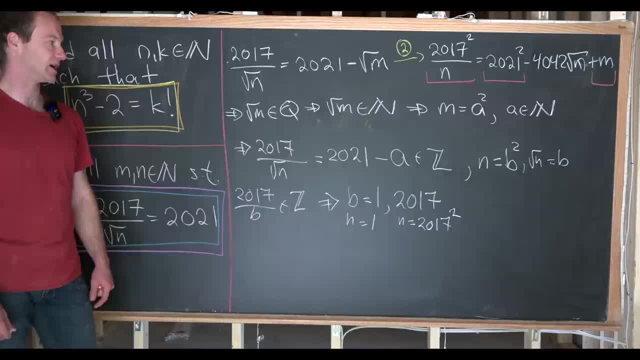 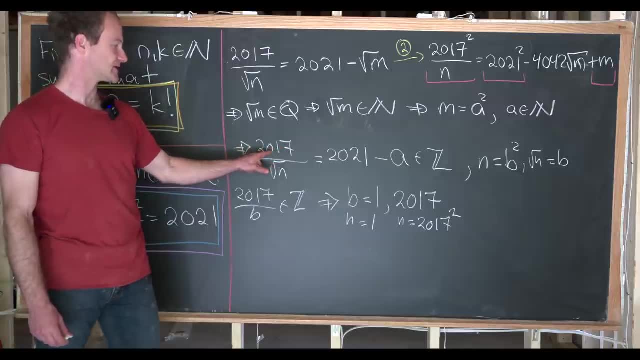 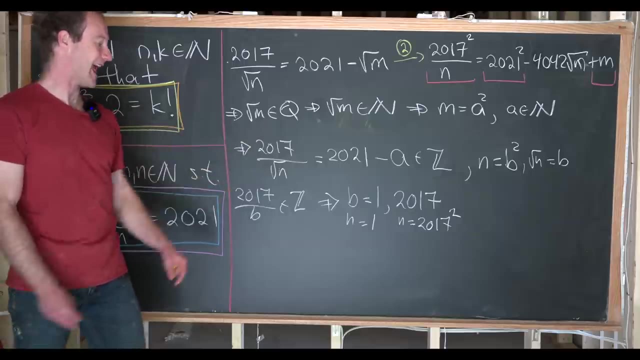 Then let's see what values of m correspond to those two values of n. So we can do that by plugging this information up here. So we've got 2017 equals 2021 minus a. We can rearrange that real quick to see that a has to be equal to 4.. 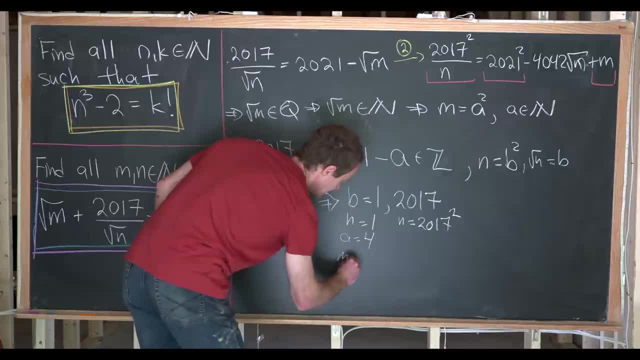 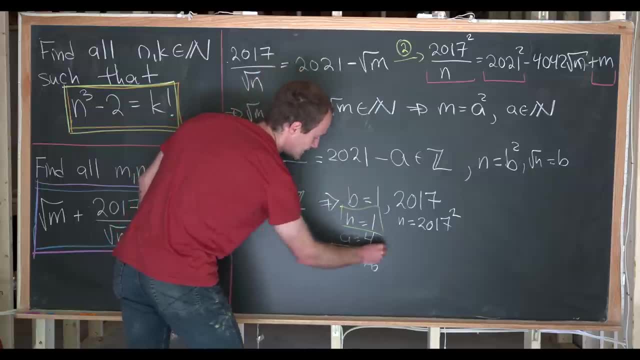 But now, if a is equal to 4,, that means that m is equal to 16. And that gives us our first pair for a solution. We have: n equals 1, m equals 16.. Now let's look at this other case.